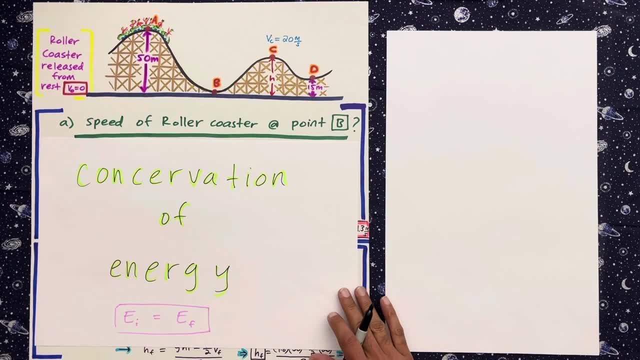 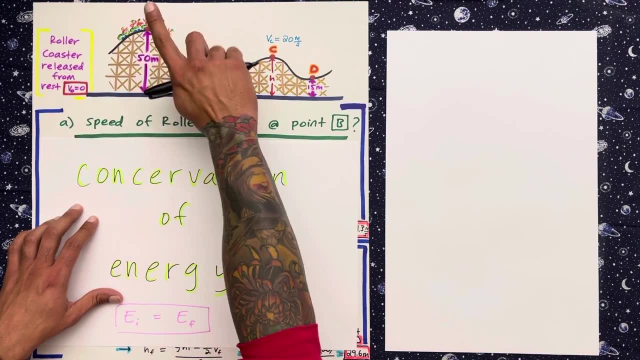 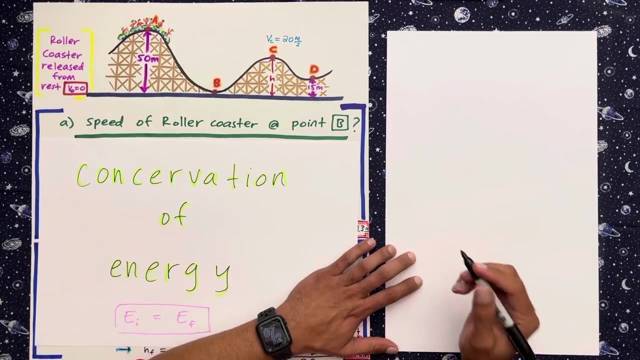 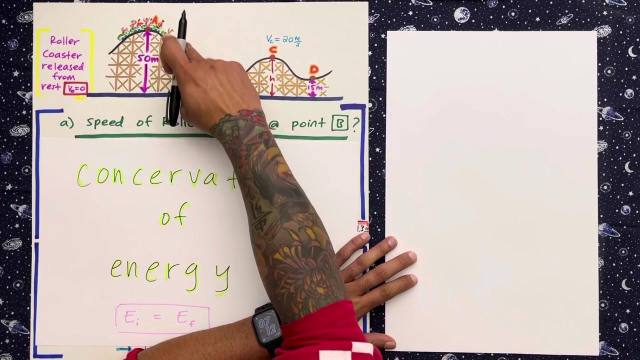 of 15 meters and what we'll look for a couple values at that point also. so, right here in the roller coaster, this is my favorite seat, right in the front. all right, let's see a couple things that we need to calculate in order to check for the speed of the roller coaster at point B. all right. 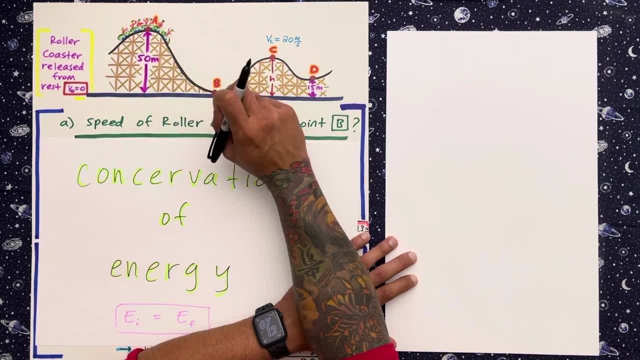 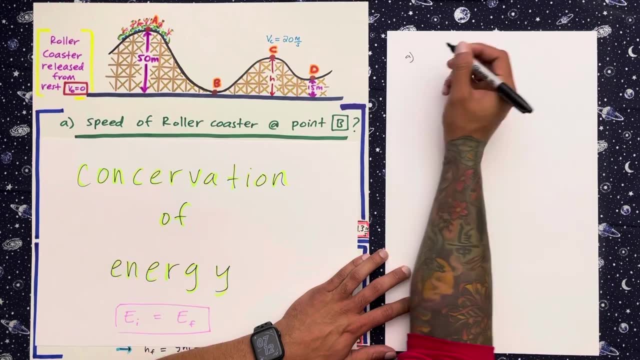 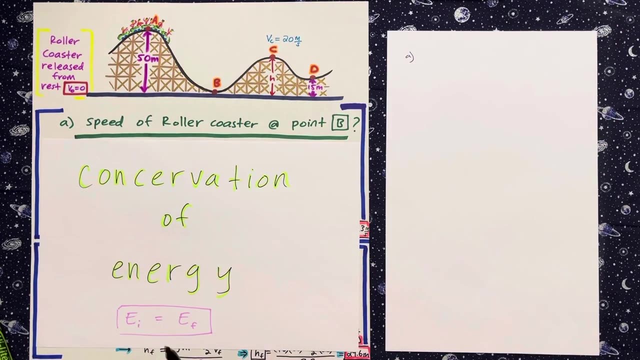 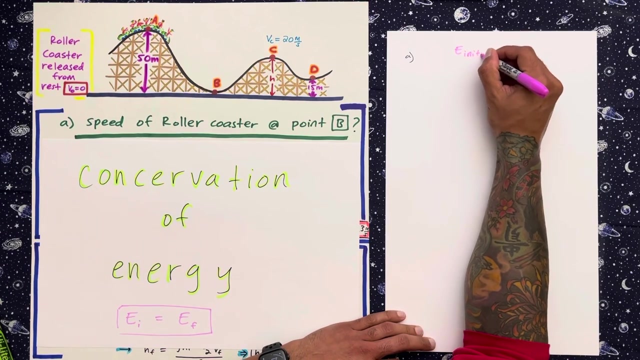 let's see how fast you can go at this point if you started at 50 meters and velocity initial was zero. okay, so for part a, and we're gonna use conservation of energy. so conservation of energy. simply, we need to remember one thing: okay, so the speed of the roller coaster is equal to the energy initial, all right. 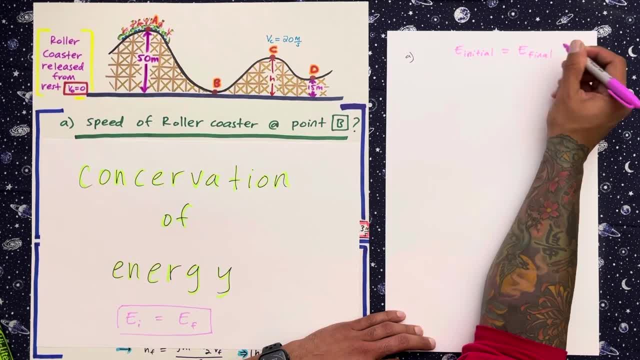 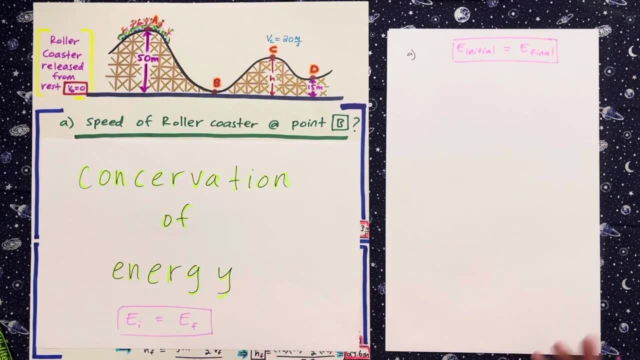 it's equal to energy final. so all the energy initially needs to equal the energy final. right, it's transformed into kinetic and potential, you know, and back and forth, but it needs to equal. so with that in mind, let's look at, let's look at what we have. so what is the speed of the roller coaster at point B? so here, okay, a. 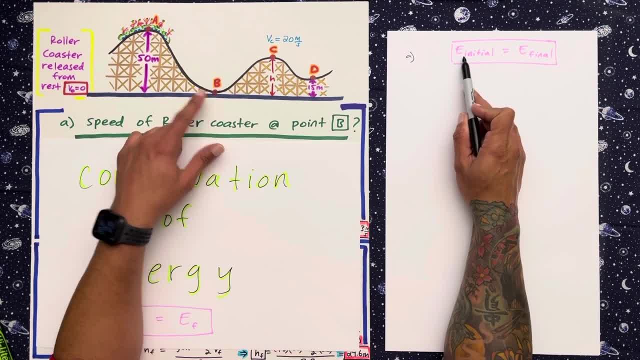 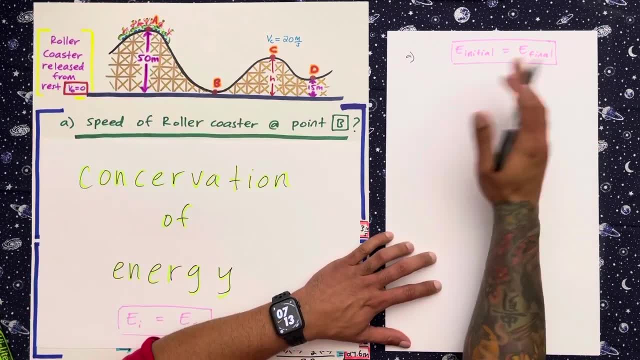 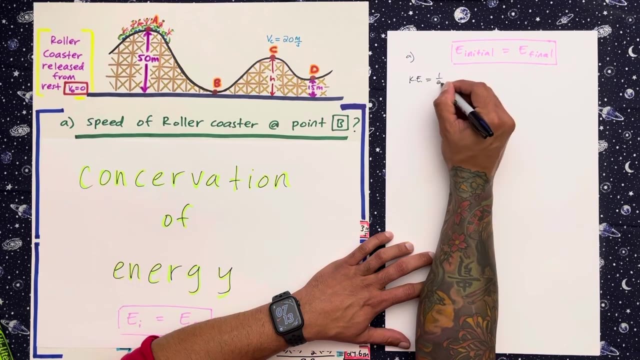 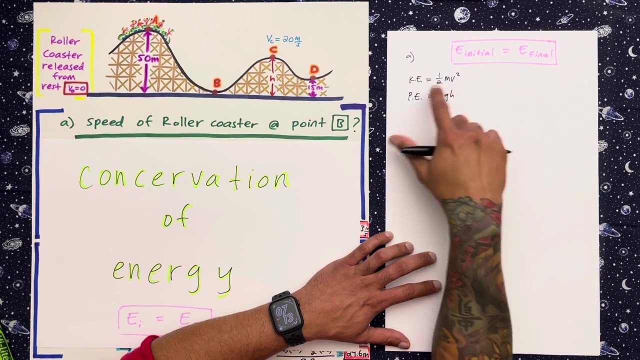 so, initially, what kind of energy do we have? well, we're all the way up here, at point a, and we have a height. so let's distinguish between the two types of energies, okay, so kinetic energy is equal to one half m v squared, and potential energy is equal to mgh. so kinetic energy. 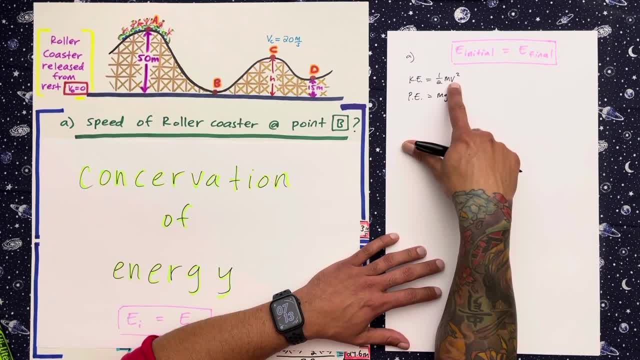 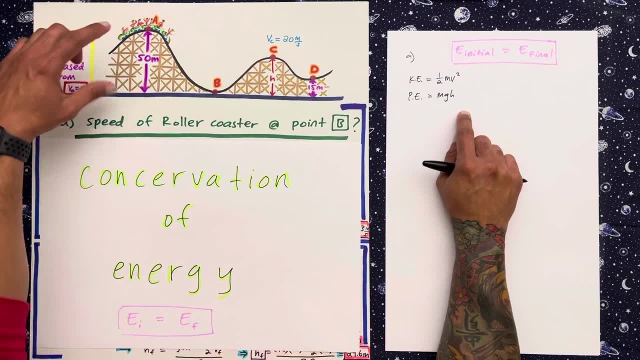 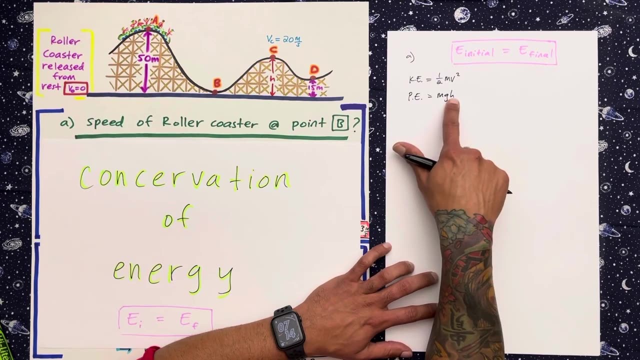 has velocity right, which allows you to calculate speed. potential energy needs a height, okay. and so if we look at the initial height at point a right, that tells us that, okay, we have potential energy, but right when we started, initial velocity was zero, so we don't have kinetic energy. 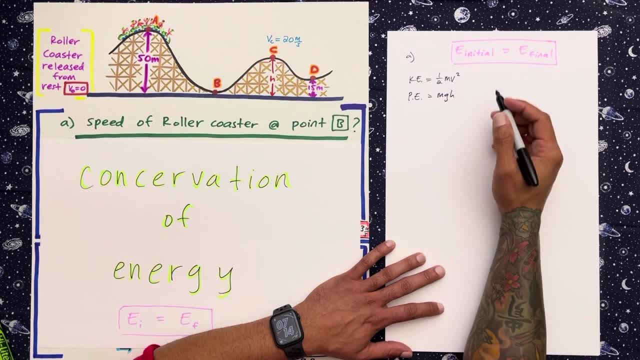 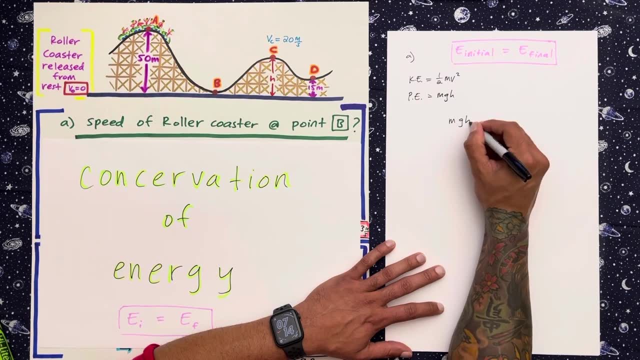 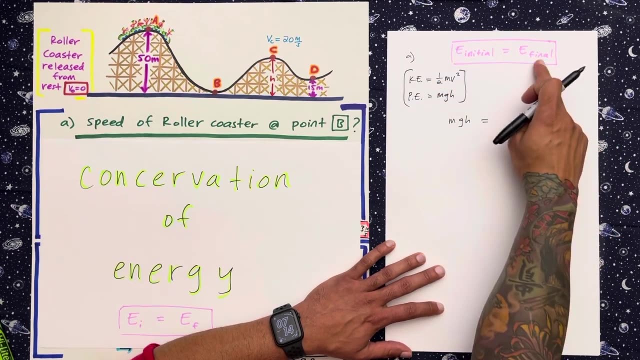 so just for initial and uh for energy. initial, we just have potential energy, so we're going to write mgh on one side. equals okay, so this is the two types, equals and now final. so our final point that we're interested in is point b. and what kind of energy? 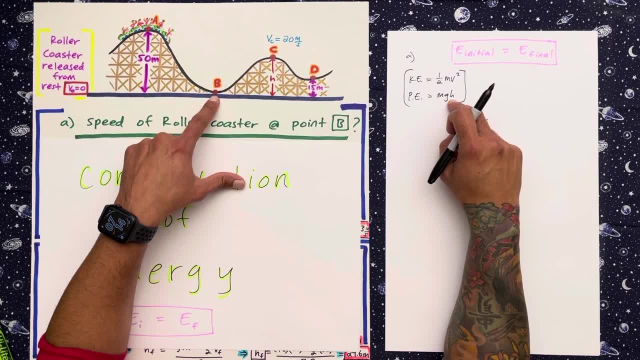 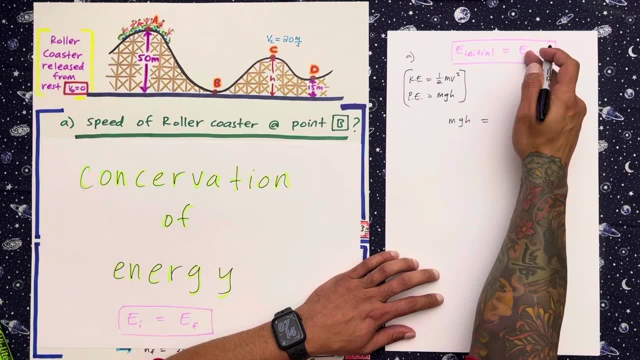 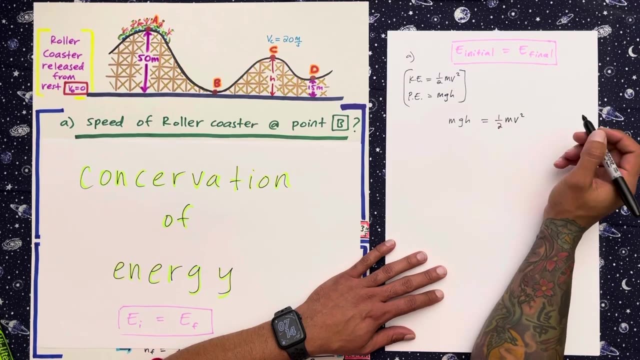 do we have down here? well, we have no height, so it cannot be potential energy and we are going to be going fast. so we're, we are going to have a velocity. so energy final first, or the point that we're interested in is one half m v squared, all right, and this velocity is at point. 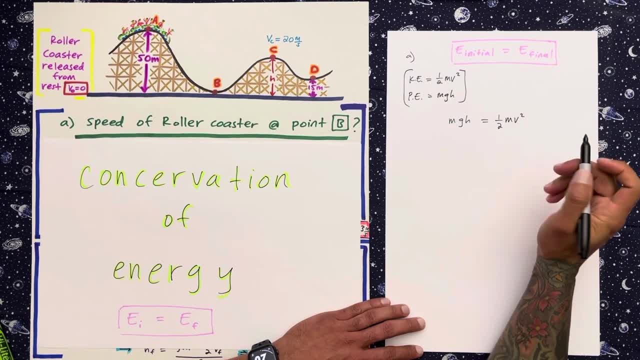 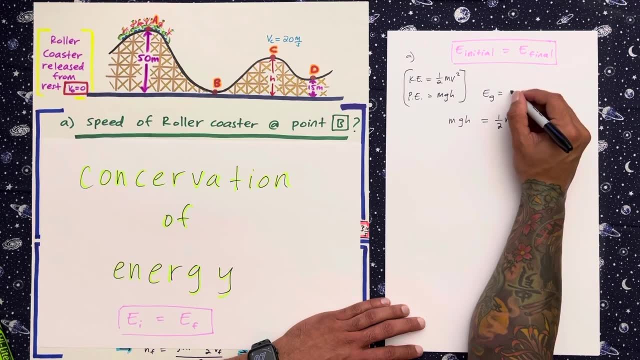 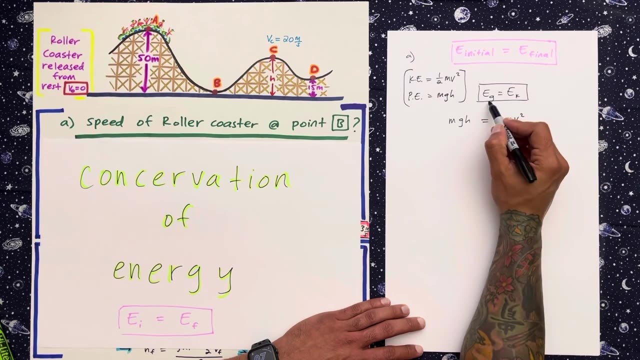 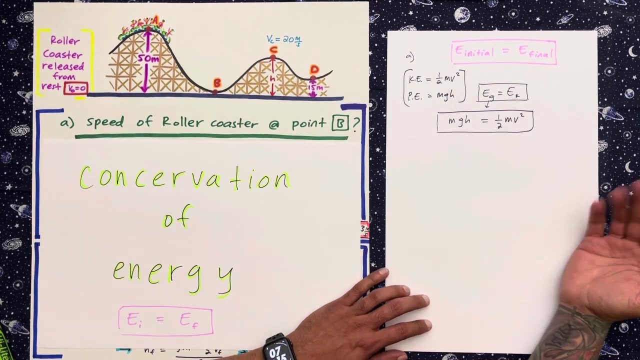 b. so now we could have also wrote on top right before we could have put energy, uh, gravity, gravitational or potential energy and energy kinetic. this is another way that you might see it, but this and this mean the same thing, okay. so now that we have this right, let's solve for velocity, because that's what we, that's what we're looking for, right? the 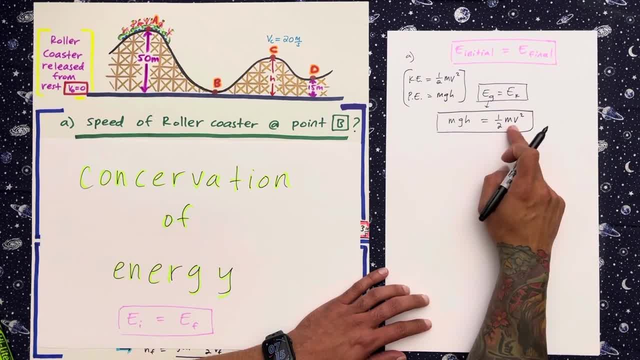 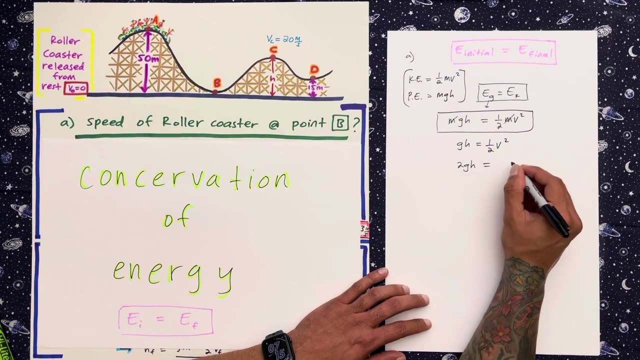 velocity at b. so we see that these m's cancel out right, because if i divide the m over here, m over m, what are we left with? we have gh is equal to one half v squared. if i pass the two to the other side, i'm gonna have two gh equals v squared right, multiplying the two to the top over here and. 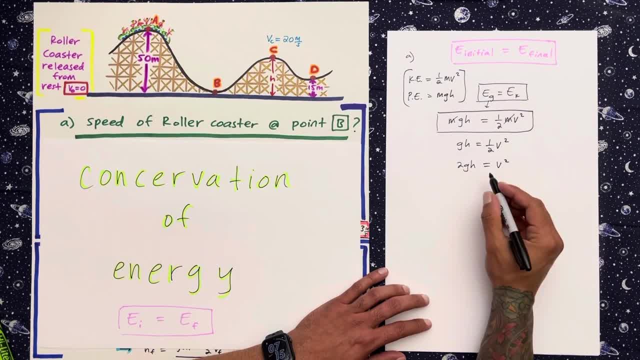 finally taking the root of the two to the other side and multiplying the two to the top over here and finally taking the root of both sides to get rid of this two. so i'm going to have v. i'm just going to put it. on the other side, v is equal to the square root of 2gh and this 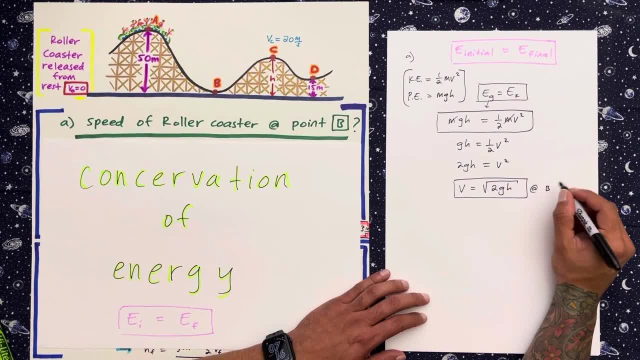 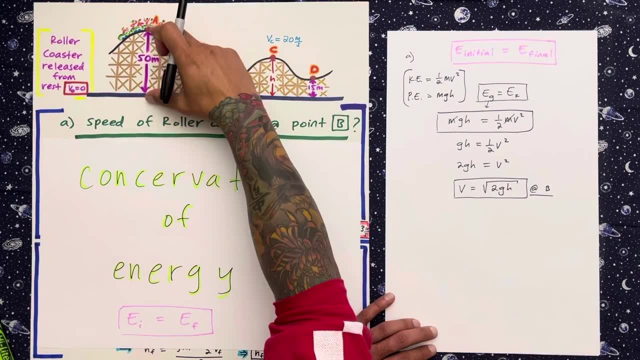 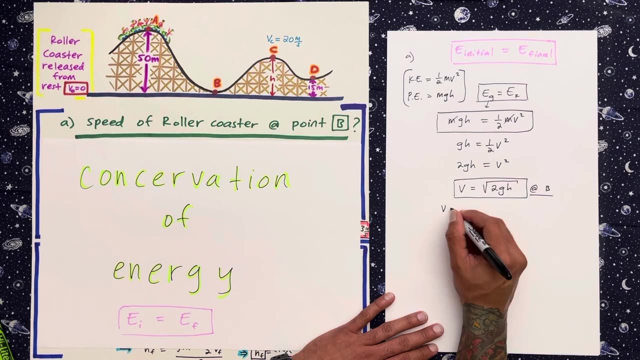 is for the velocity at b. okay, so let's put in the numbers. all right, initially we were given the height, which is what we need. we know g is gravity, so we know that we're going to have. velocity is equal to 2 times 9.8 and the height is 50.. okay, so putting that into the calculator. 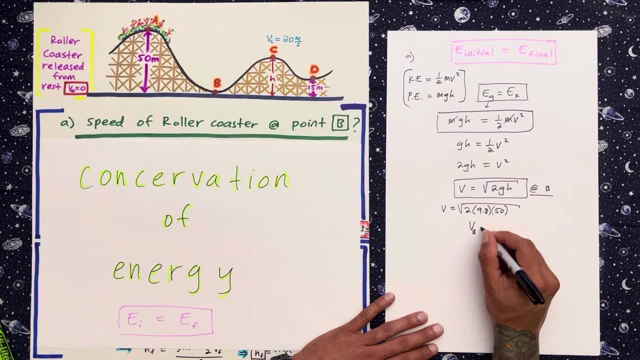 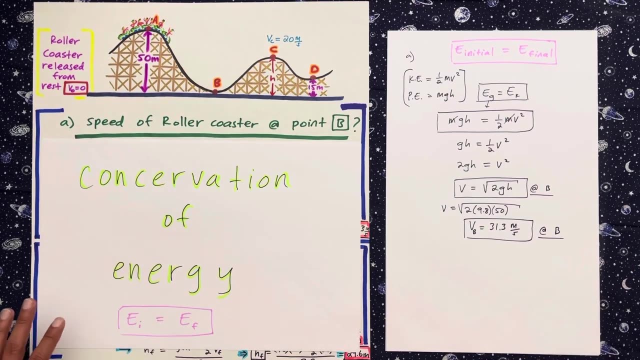 we get velocity at b. i'll denote it with: b is 31.3 meters per second. remember? that's the units for velocity. okay, so this is the velocity at b. all right, weわ heihin, we are moving on, and now let's. Okay, so moving on. 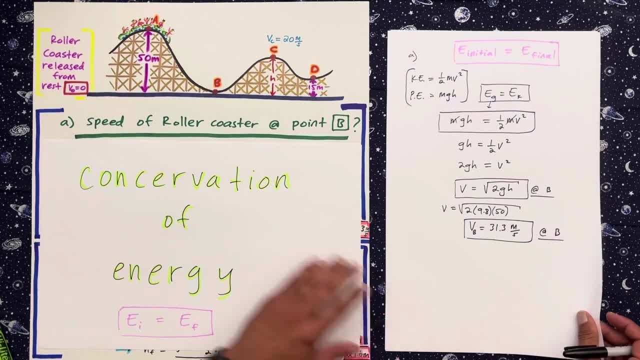 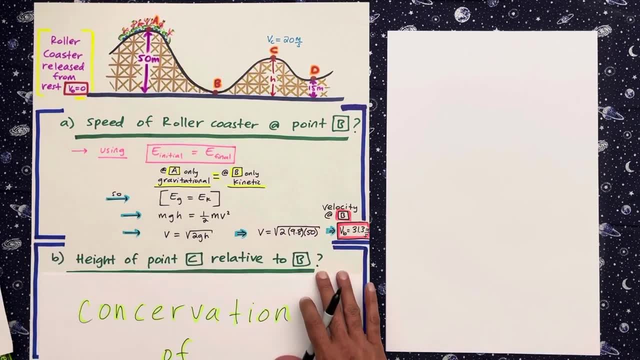 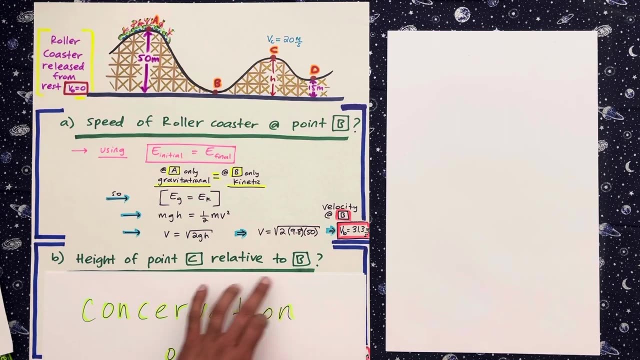 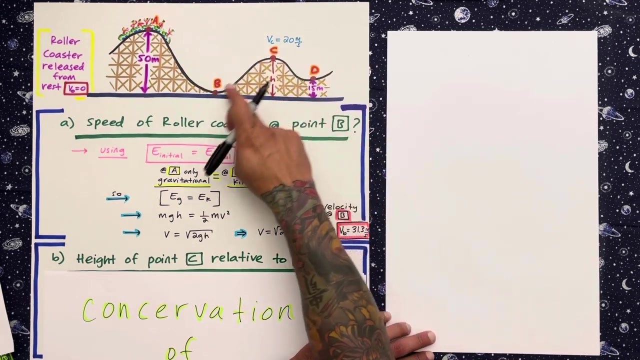 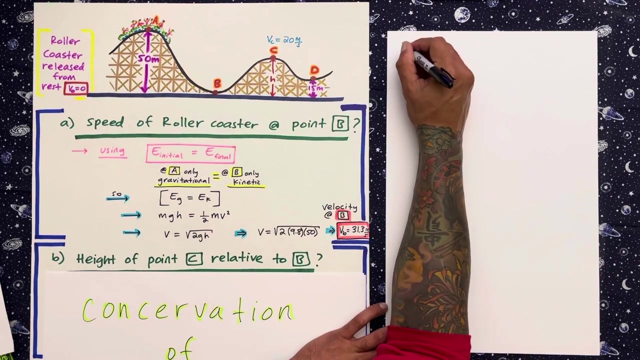 let's do now- i'm going to put this over here now- let's do part b. okay, we have height of point c relative to b. okay, so height of point c, which is this h right here, relative to b, so we're we're looking a direct comparison back to b, which was on the ground, and c, which is up here. so let's do part b. 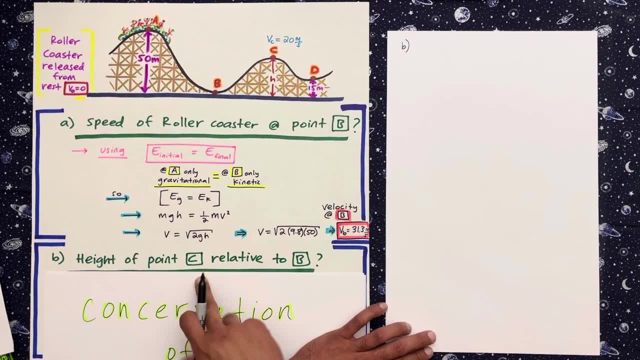 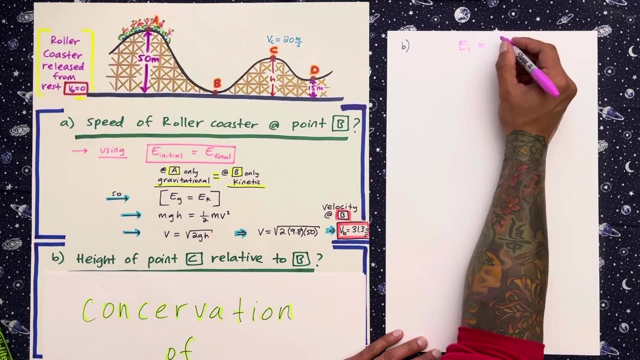 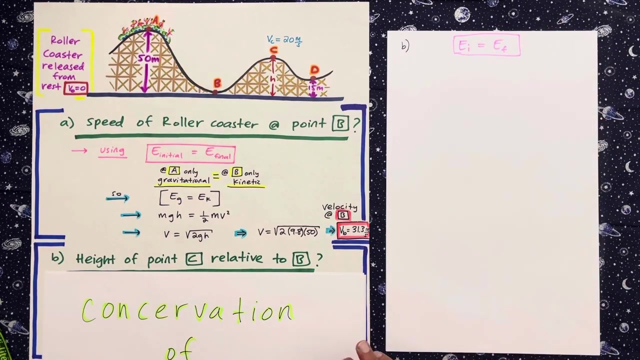 we're going to be looking for the height of point c relative to b. all right, so again, before anything, right, right. when we know we're doing, uh, conservation of energy, we start off with always, energy initial is equal to energy final, all right, always, okay, you can even, you can even do, instead of uh trying to guess where everything is at. 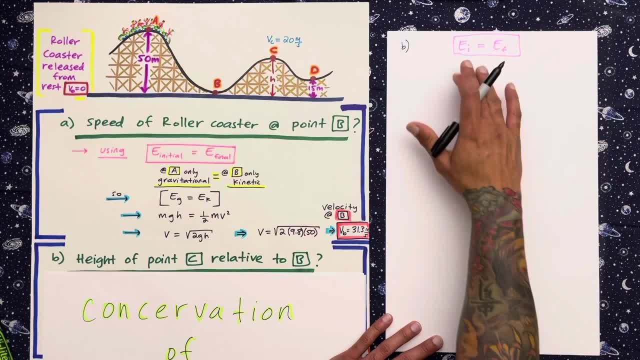 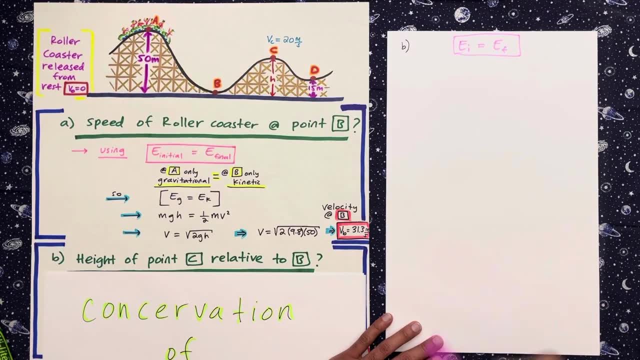 um. in other words, instead of trying to understand, oh energy, what energy do we have here, what energy do we have here? write the whole formula out, so that way it's always apparent to you: energy initial is equal to energy final. all right, so we're going to be looking for the height of point c. 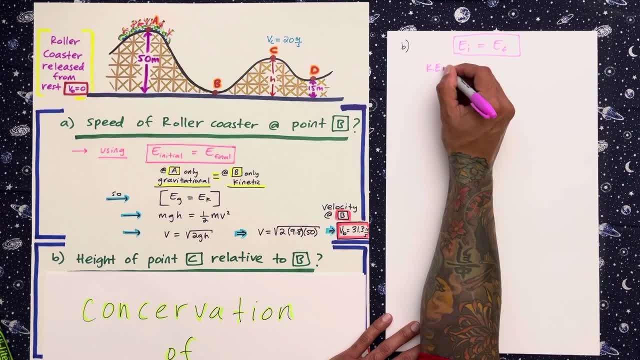 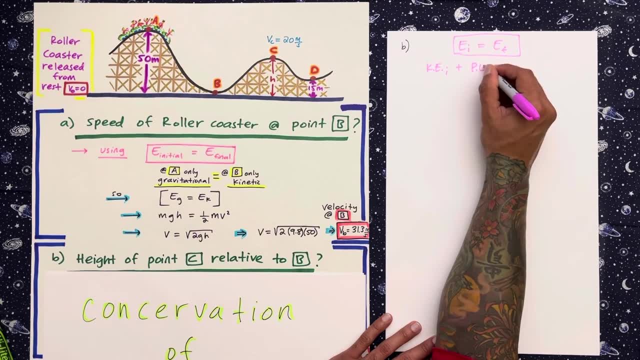 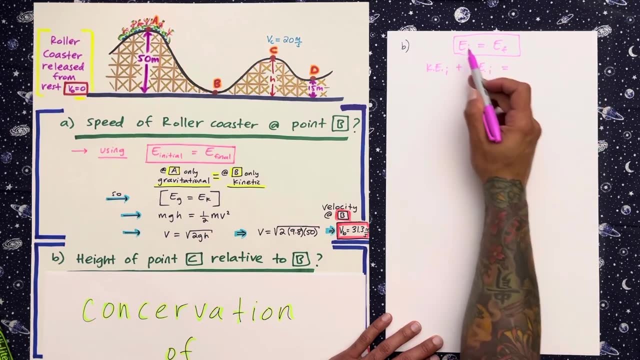 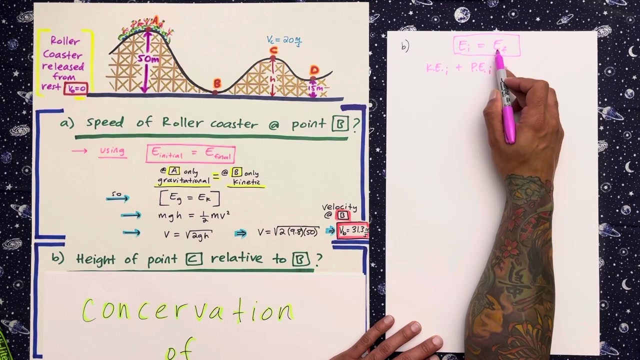 energy initial means we're going to have kinetic energy, right, initial? oh exactly, okay. plus potential energy. initial is equal to: so this whole side here is just for energy initial. you have to have kinetic initial and potential initial, then you have to do the final energy, so you have kinetic energy. 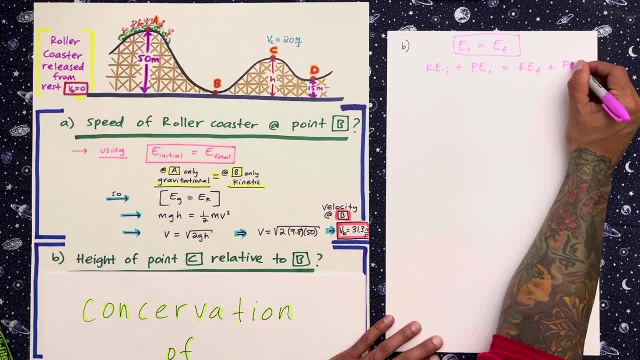 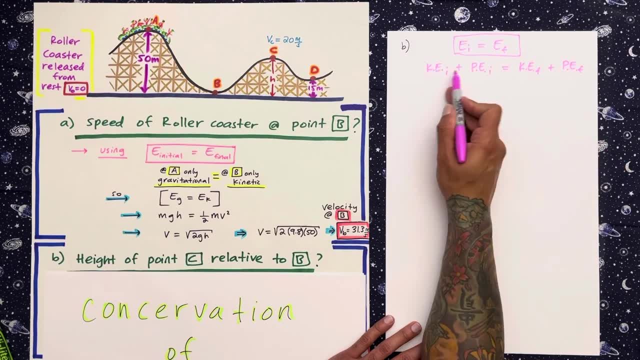 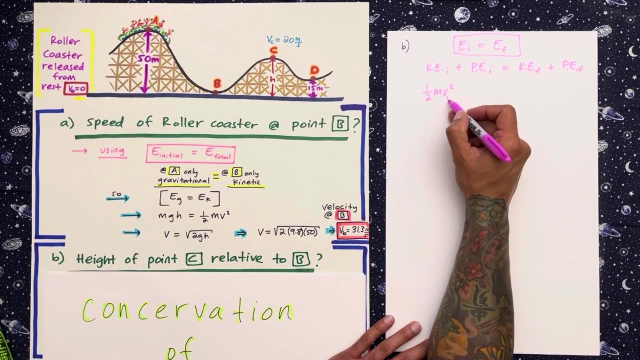 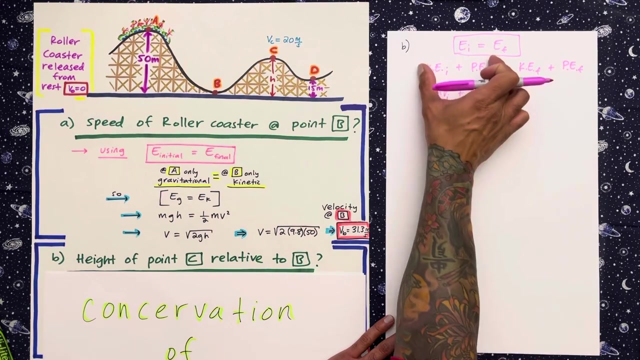 final plus potential energy, final. okay. so one more uh, one more simplification. we know what kinetic energy is, so it's a one half m v squared and that's going to be velocity, initial right plus m, g, h. that height is going to be the initial height, right, because we're in the uh initial side. 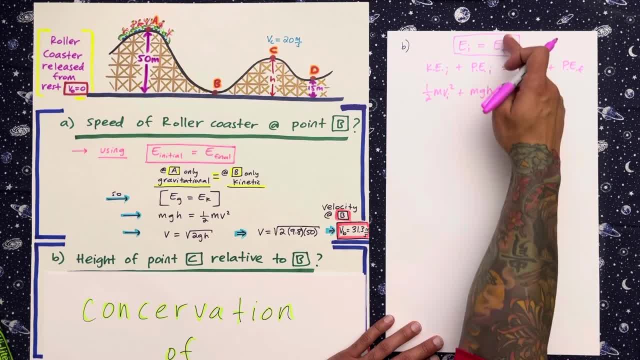 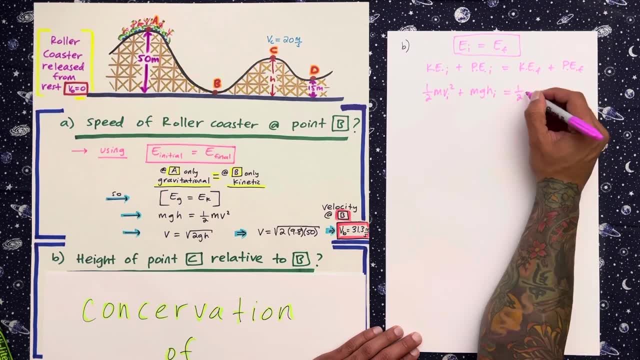 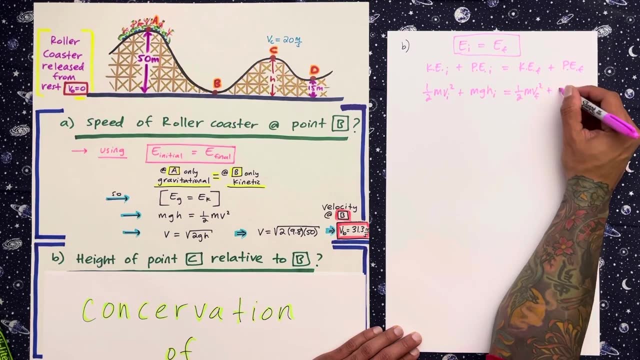 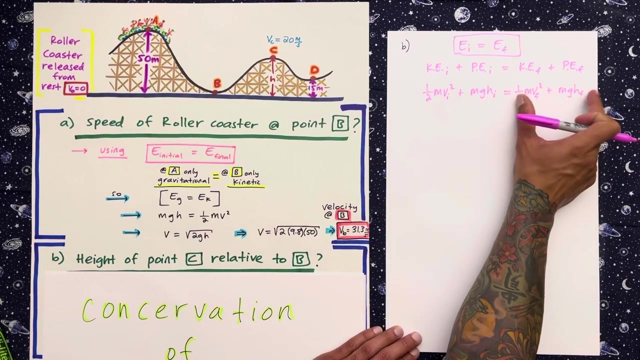 of the equation now equals. now we're going to do the final side of the equation and here we got one half m v squared, final right. that's the final. and plus m g h height, final. okay. so initial side and final side: okay so now. now we can look at what we need and what we don't have. 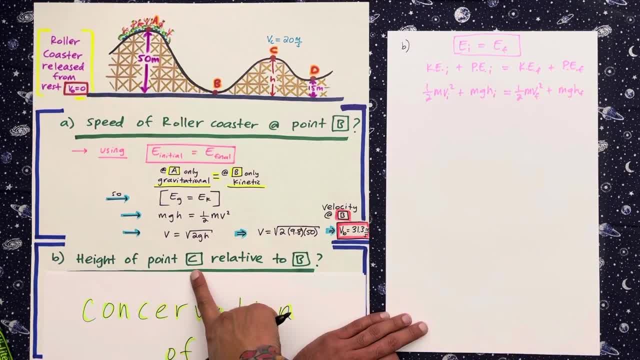 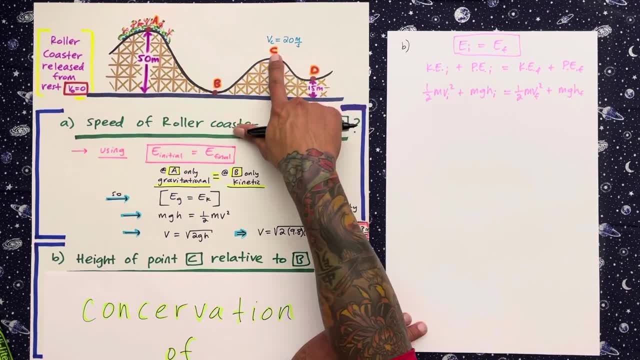 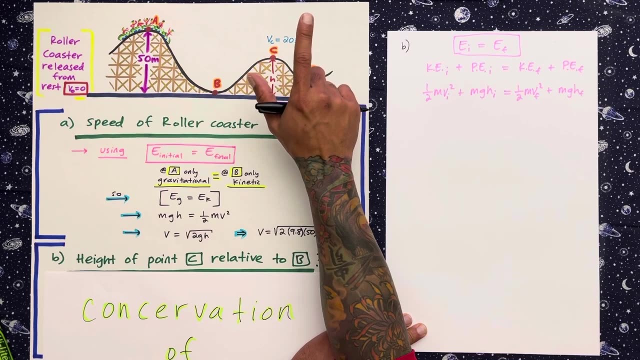 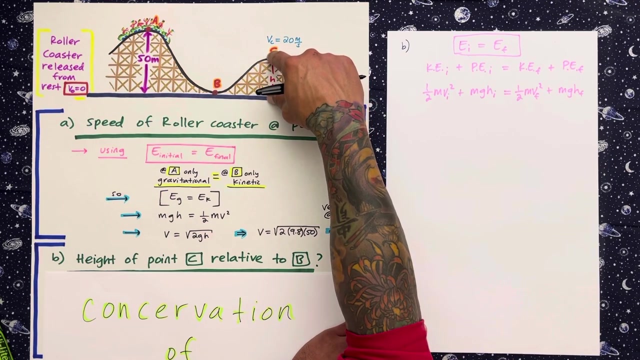 so first, let's take a, let's read the question again: the height at point c, right relative to b. so this is what we're looking for. so it tells us that at c we know that there's already a velocity. okay, so, um, we're gonna, we're gonna look at this part here and we have an initial height. okay, so we don't have an initial. 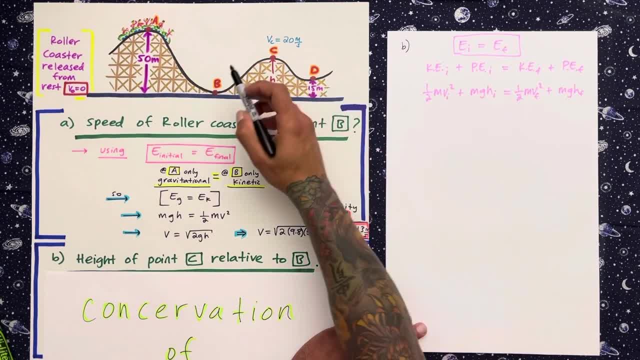 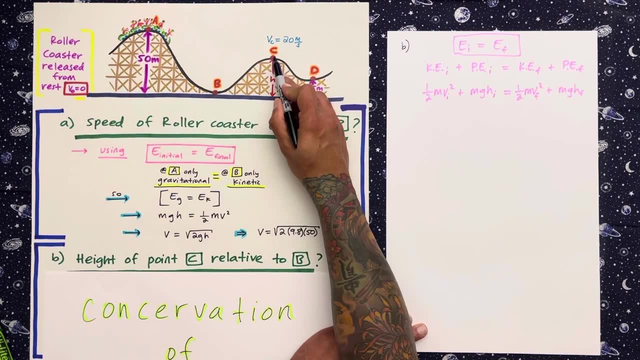 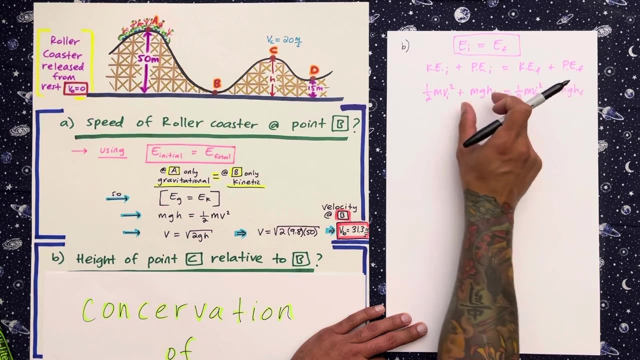 velocity, because initial velocity started off here. all right, we're gonna do straight the final velocity, which is vc, because we're going to calculate this height. so the that velocity here is going to go on this side. all right. so we have height initial. that we're going to keep. so this is zero, right, because here we don't, we're not starting off with. 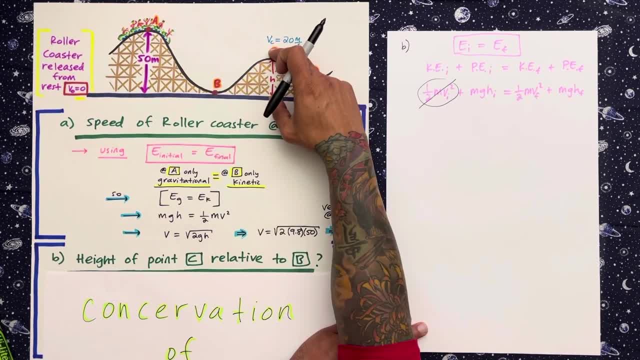 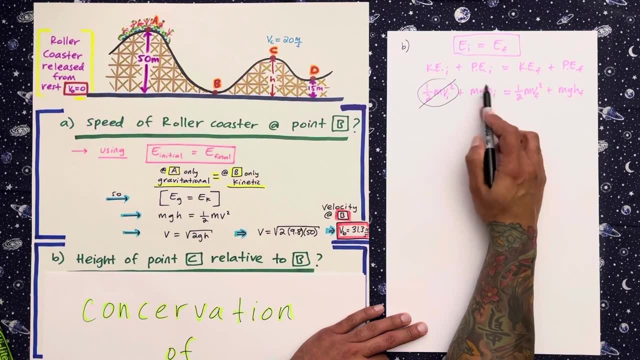 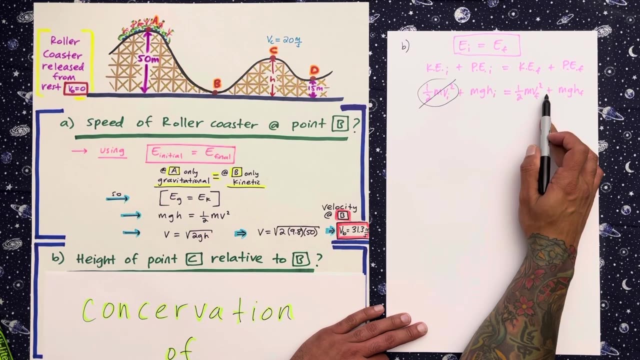 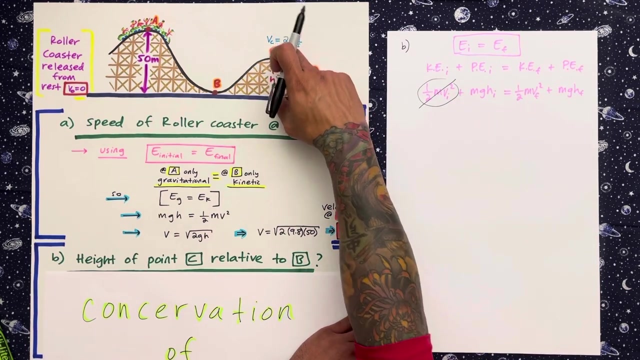 a velocity we're just starting off with. we want to know here the height, so for that we're going to use this velocity, this height height initial. okay, we're going to leave that there, and over here we have one half mv squared final. um, we do have a velocity right final and mgh final, so obviously this is the one we're looking. 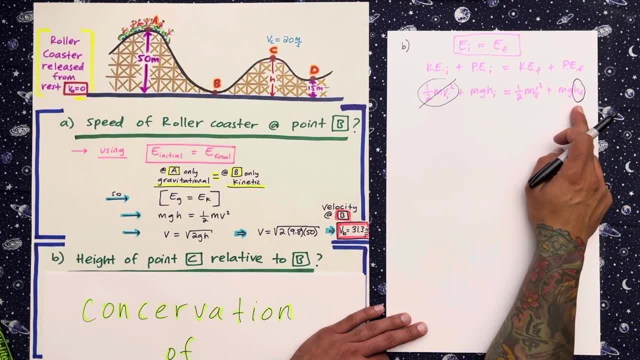 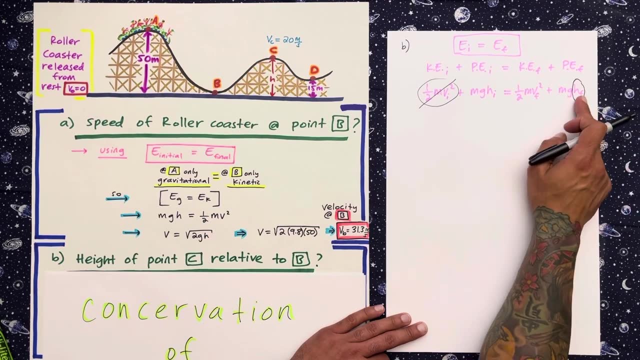 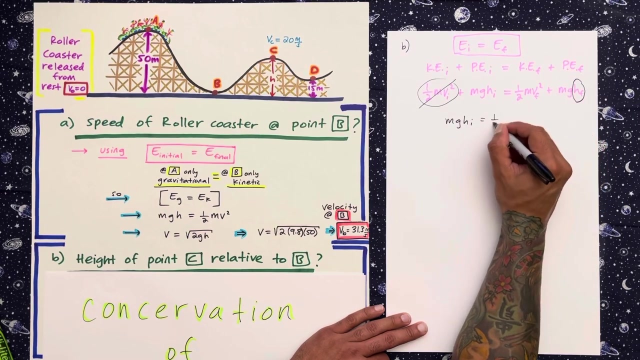 for right here, the height final. okay, so let's rearrange everything to have high final in our. our equation equals something else, okay, so in other words, let's solve for h final. so what do we have left? we have mg. h initial is equal to one half mv squared final plus. 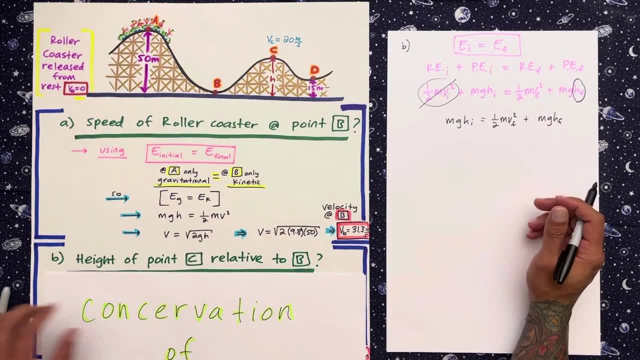 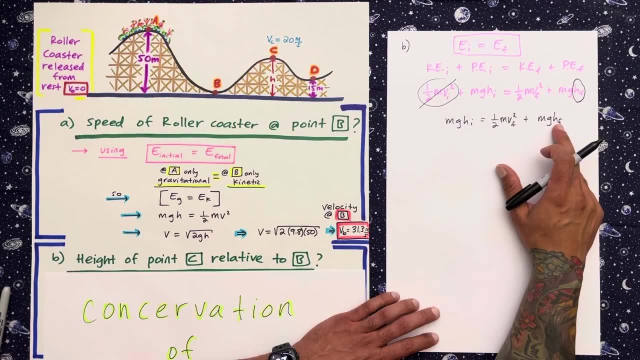 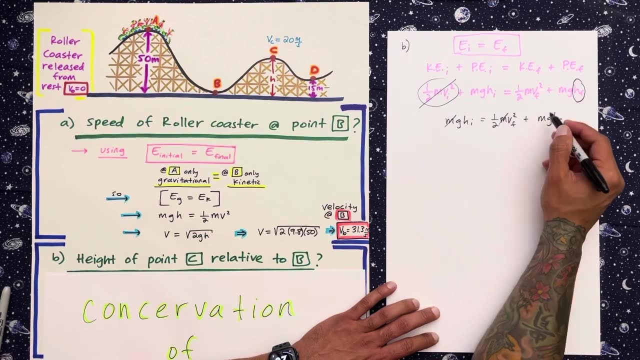 mgh final, okay, and so what we're looking for is height final, so the height of point c relative to b. so we're looking for height final, and what's that going to be? we have, um, all the m's cancel out, right, because we divide by m for everything, and i want to put this whole thing on the. 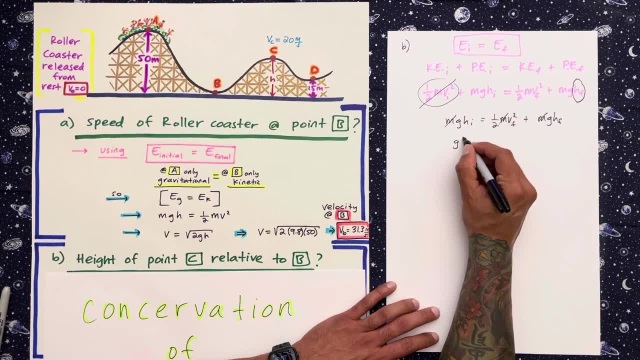 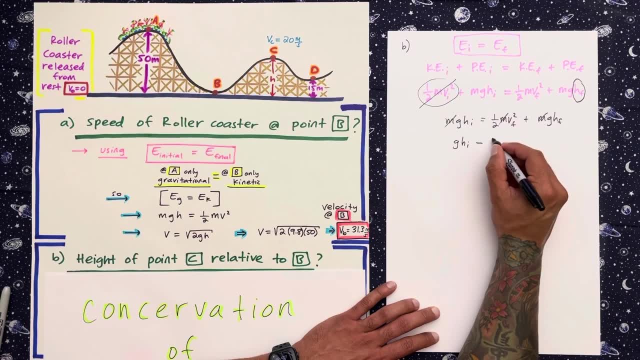 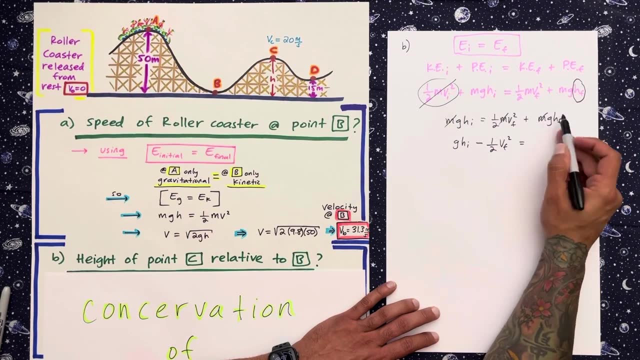 on this side, so i'm still going to keep this. i have g height initial. if i move this over to the other side, it becomes minus one half velocity final squared and this side stays right there. so that's going to be gravity h final. okay, so let's. 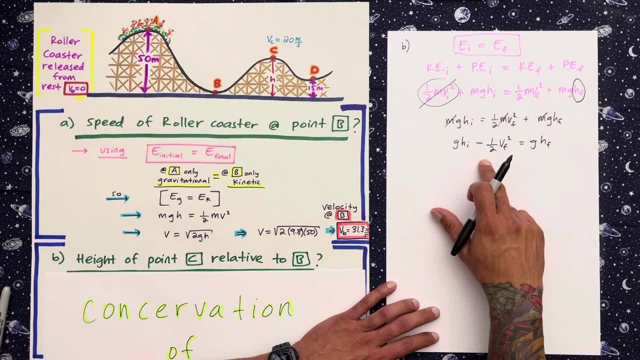 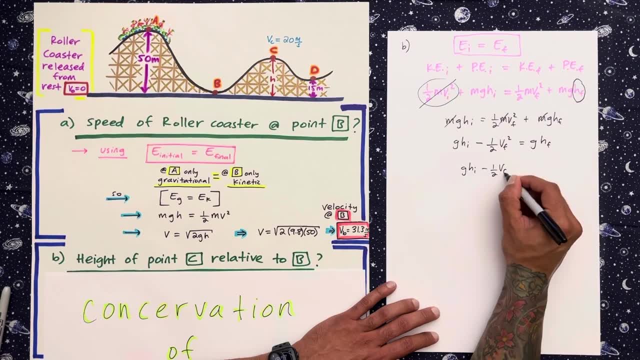 do one final step: get rid of the gravity. we're going to divide it to the other side. so i'm going to keep all this on this side the same, to make things a little easier, and then i'm just going to divide everything there by g, h, final, and that's what we're looking for here. okay, so we have all the numbers, um. 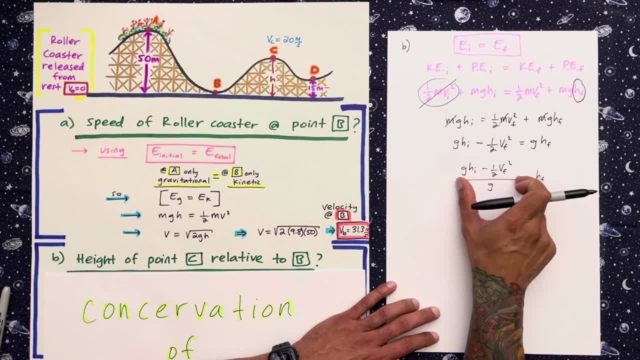 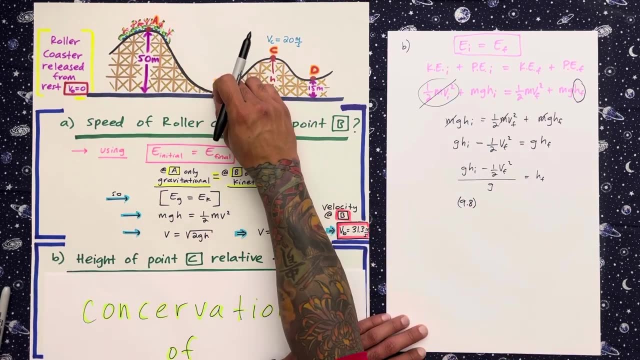 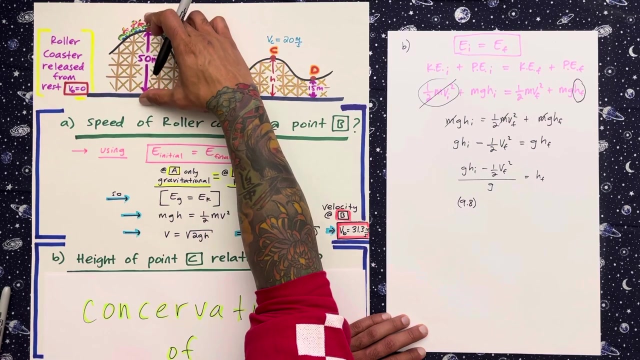 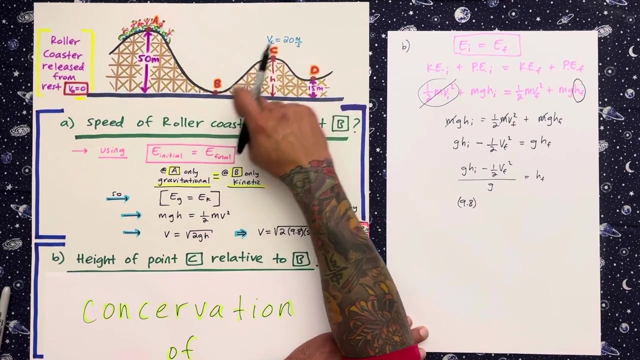 that we need. all right, let's plug them in. so gravity, which is 9.8, right, height initial: okay, so height initial was not from b, which is why we made velocity initial zero. we're looking from here right to here. so the height of c relative to b right, which is this one. but we have to do. 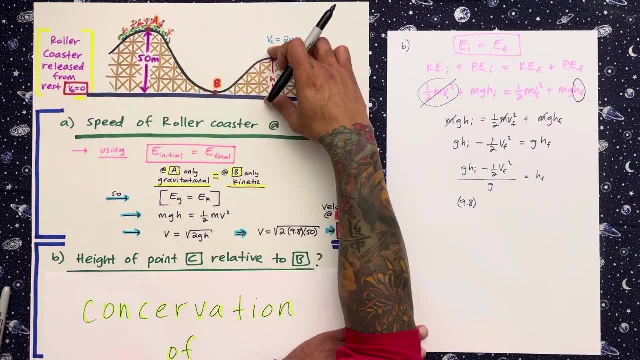 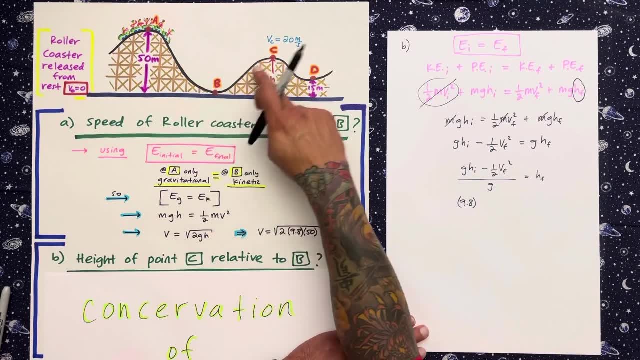 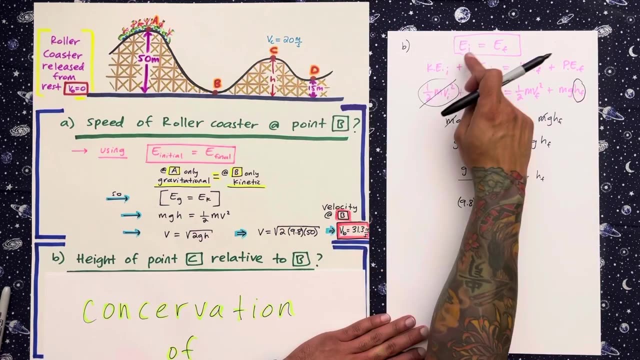 the energy from the initial to the final thing that we're looking at. so don't let that confuse you, because this says relative to b. that just means that you know we're looking at the height. that corresponds from here to here, but always when we're doing in. 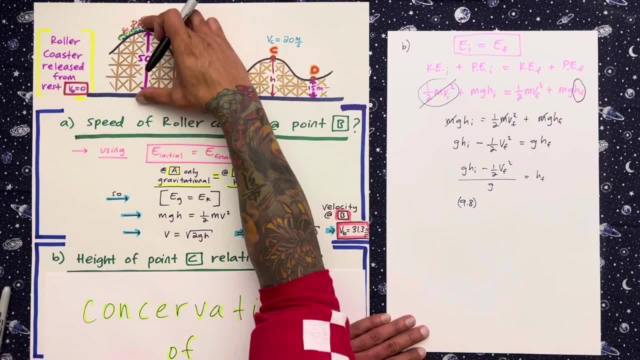 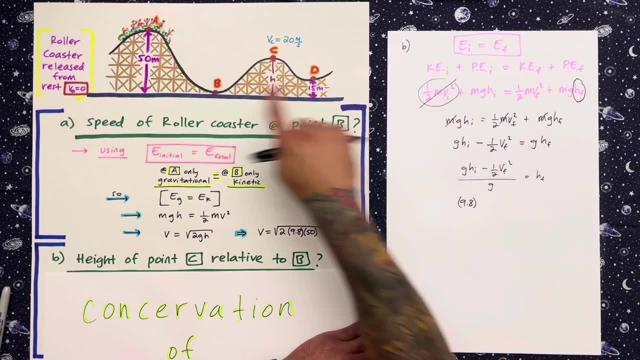 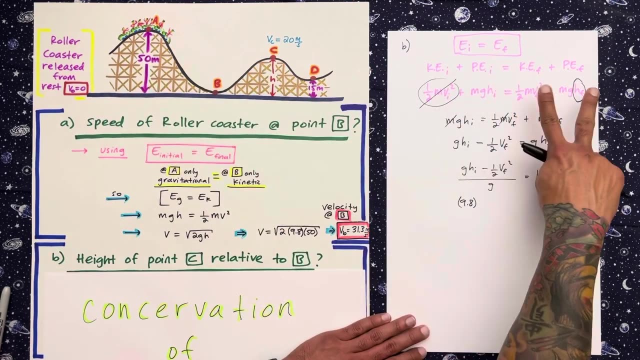 initial energy and final energy. we have to look at the initial energy and the initial energy. we did not have a velocity initial, because it was zero, right, we have an initial height which is 50. so that this side is good. and now this side here corresponds to: 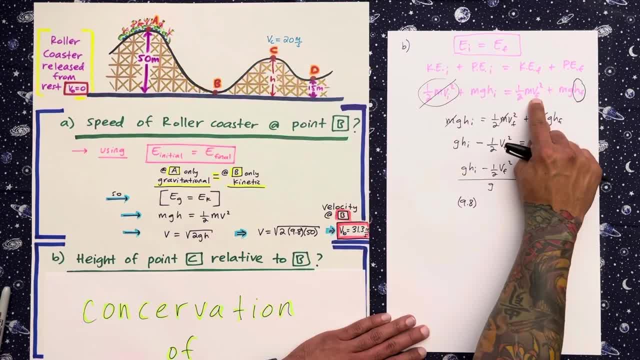 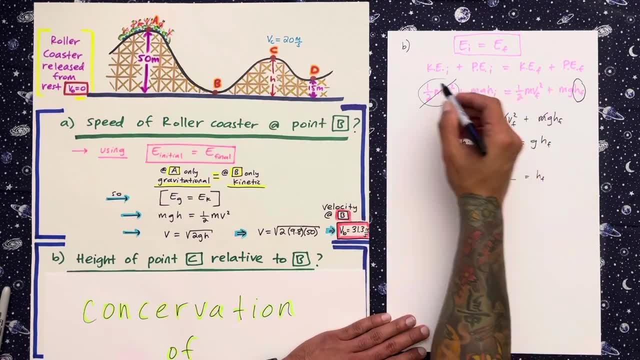 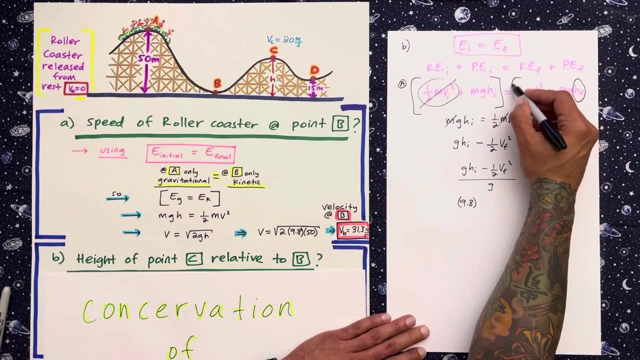 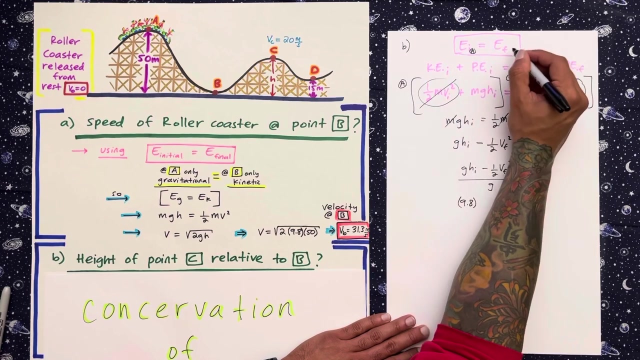 um, everything that's here at c, we have a velocity final- yes, we do, and high final. that's what we're trying to find. so, in other words, everything here on this side corresponds to point a and everything here on this side corresponds to point c. so energy initial of a energy, final of c, okay, so we're going to bring that down and we're 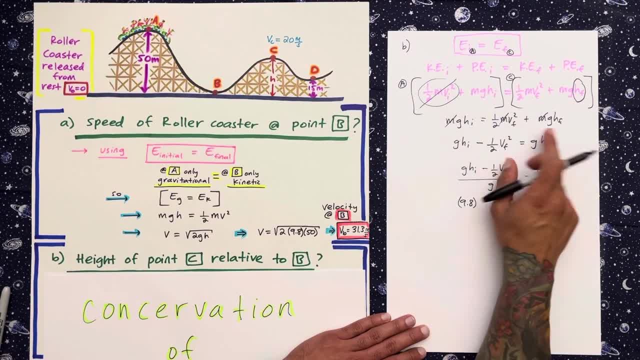 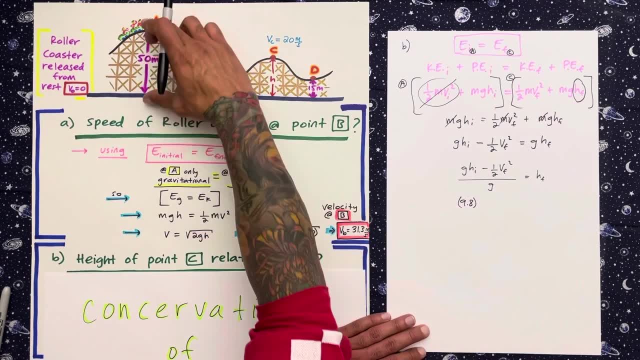 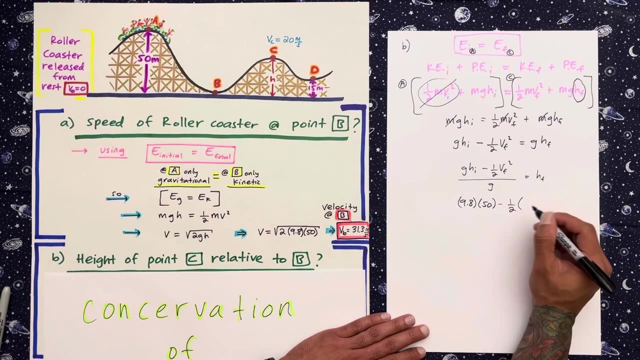 solving now. right, this got cancelled out. we have all these values and we're solving for height final. okay, what is height initial? well, i had initial 50 right minus one half velocity final, which is here. so initial final. we got 20 meters per second right and that's squared, all right, and everything divided by 9.8. okay, perfect. 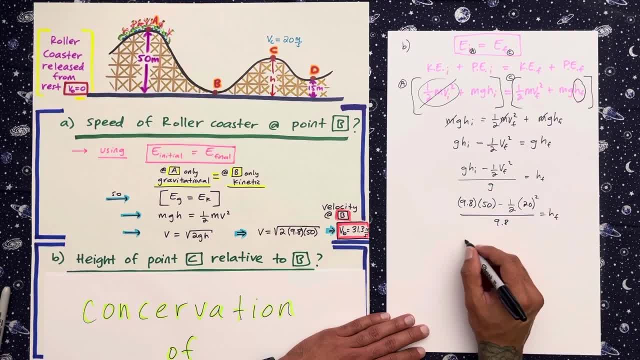 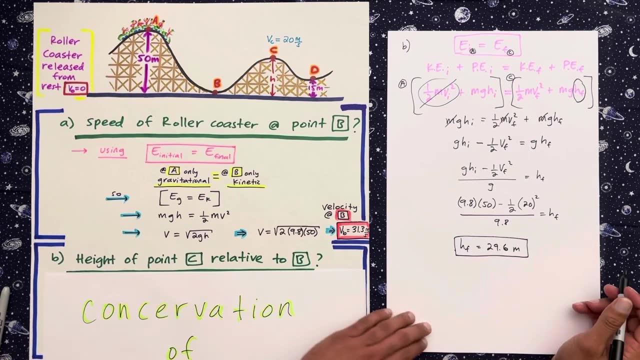 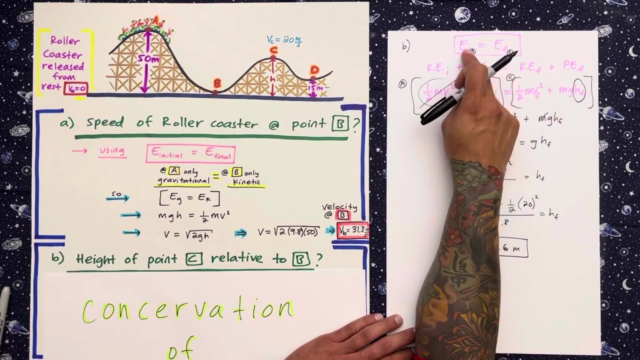 so this is equal to height, final. let's put that in the calculator and i'm getting 29.6. okay, meters, so the units is meters for height, all right. so again, remember that when we're doing initial energy, final energy, you need to go to initially what happened, what energy we looked at, right, so don't let the problem confuse you by. 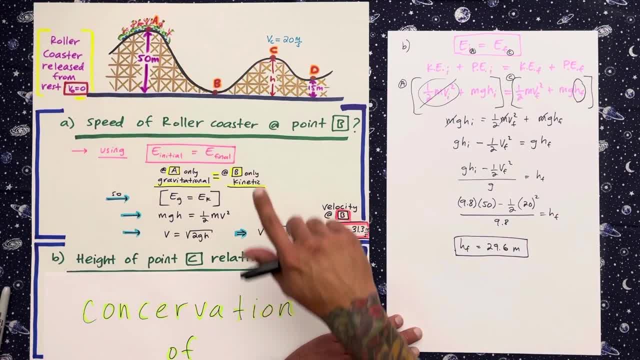 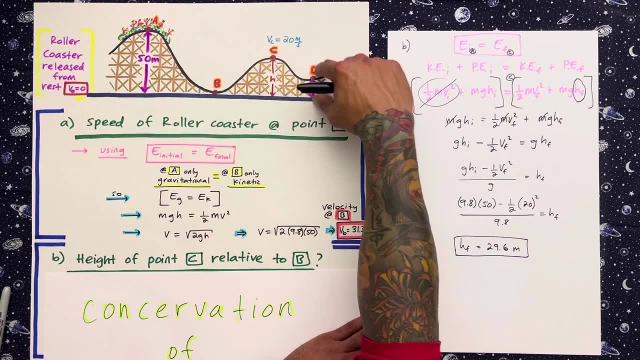 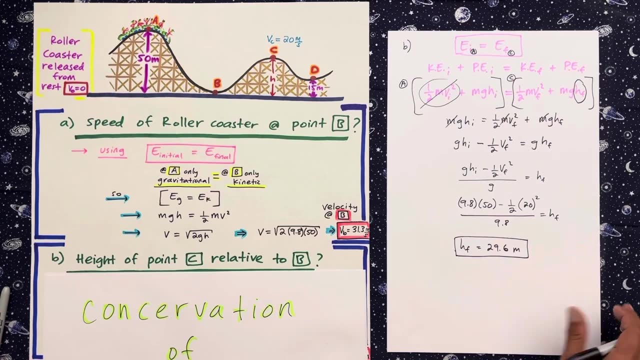 relative to be. that's, uh, that's on purpose, you know, but what you need to focus on is the initial energy from the beginning, and then wherever we're stopping at is going to be the final energy. okay, so now let's take a look at part c and see if we can tie in, tie in the rest of this. 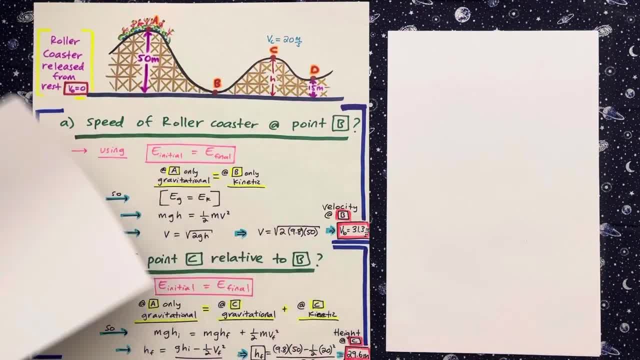 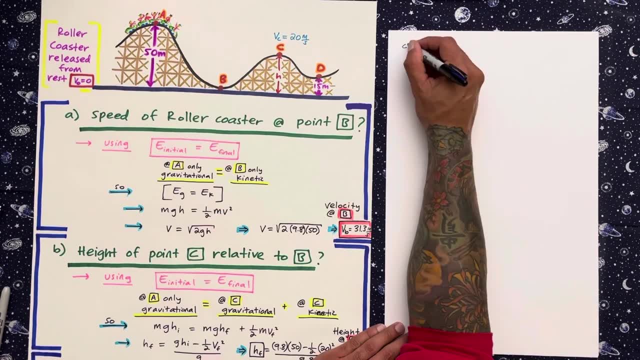 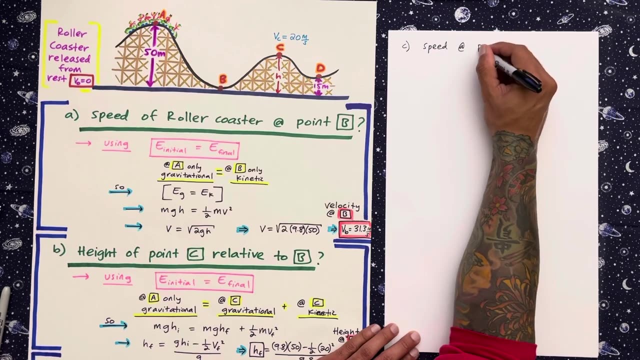 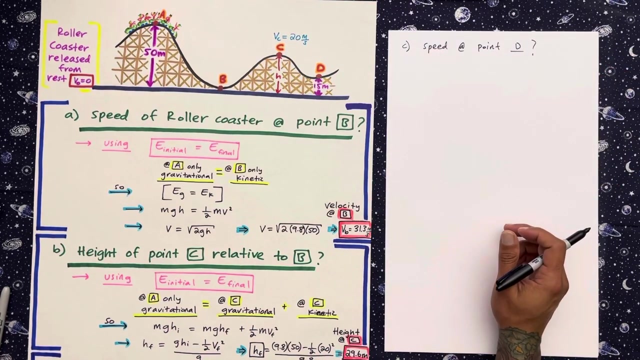 okay, so for part c- um, i won't be able to see it here, but let's uh. okay, so for part c. we want to know the speed at point d, so that's for part c. okay, so now let's take a look again. what do we start with? 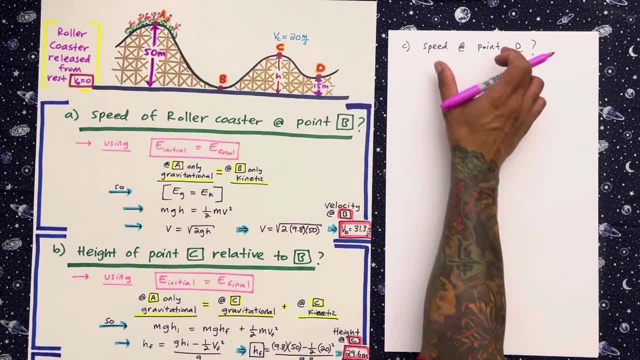 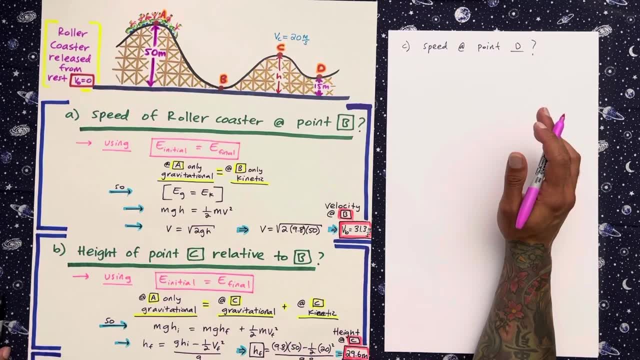 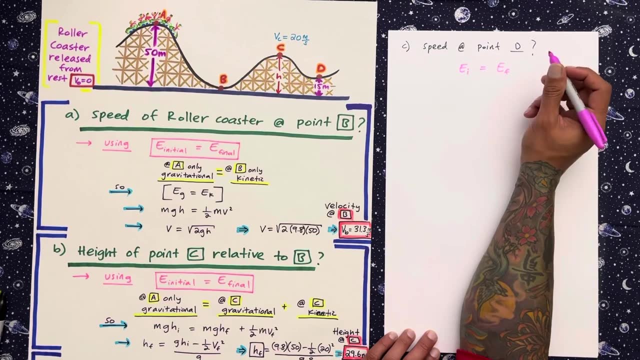 right, right, right, right, right, right, right. we're using conservation of energy. we want to know the speed here. right, we know the height, we don't know the speed. so first of all, before anything starts, conservation of energy equation: right, energy initial is equal to energy final and, to be a little more specific, right energy initial. 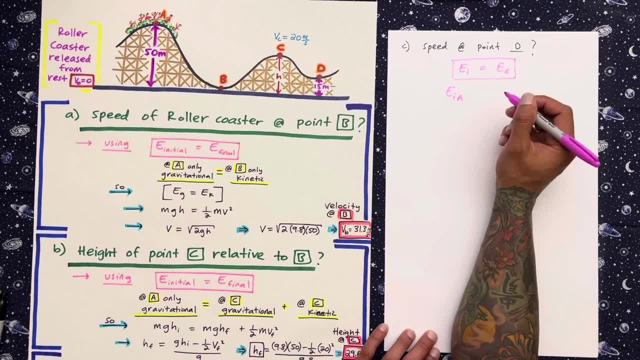 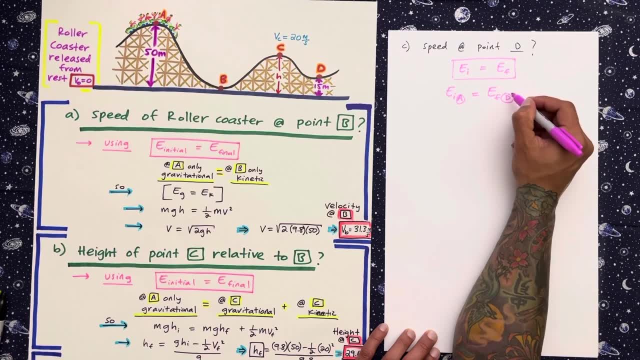 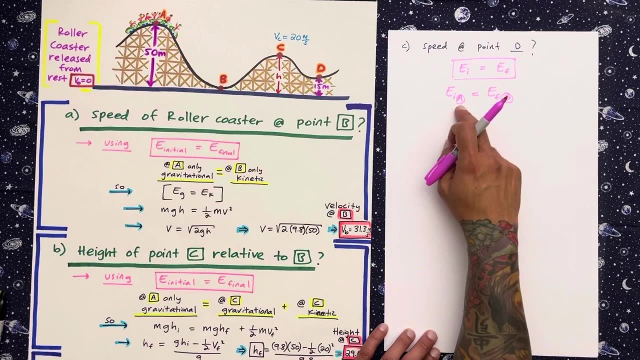 at point a right circle that is equal to energy. final, at point d, because those are the two things that we're interested in. we're always going to start at a, so this is just like the previous one. we started at a right um, all three of them. we started at the initial and then wherever we're. 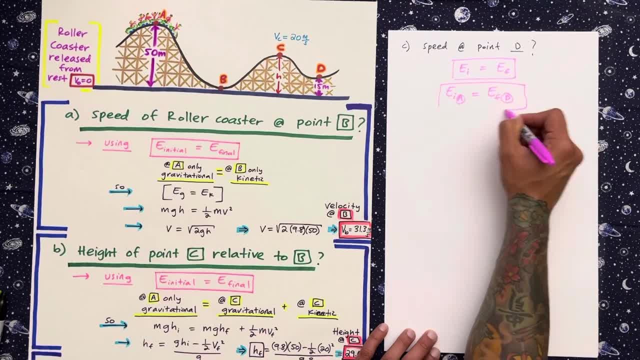 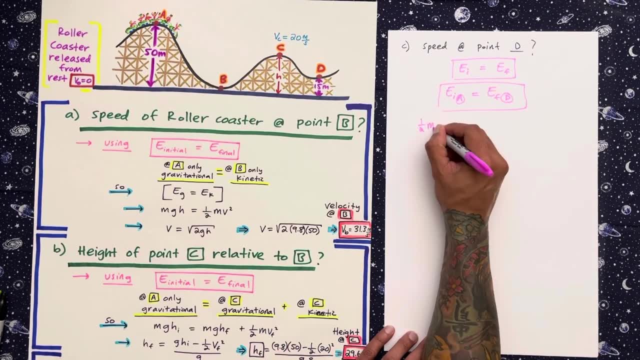 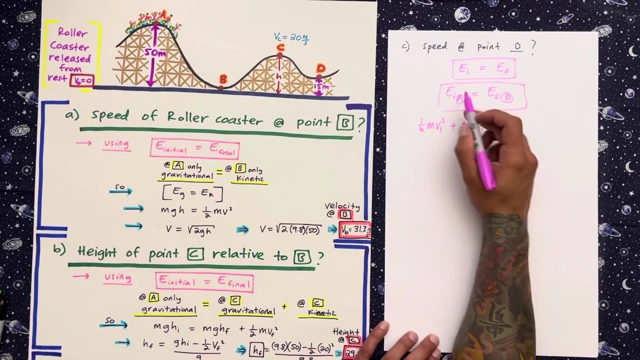 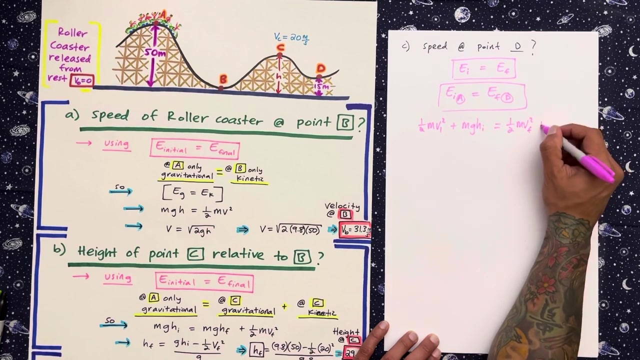 looking at is going to be our final energy. okay, so now, um again. here we have one-half mv squared initial plus mgh initial right that's for this side equals. now we're going to do the final one-half mv squared final plus mgh final. all right, so let's figure out what. 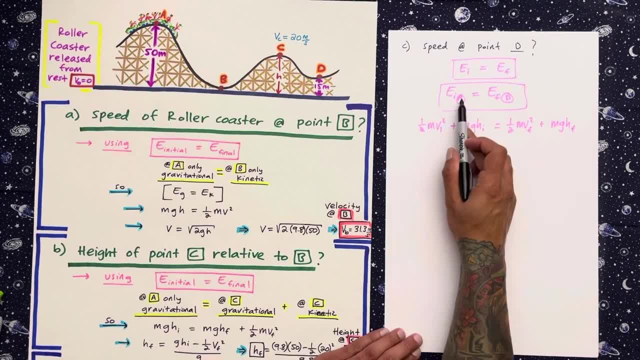 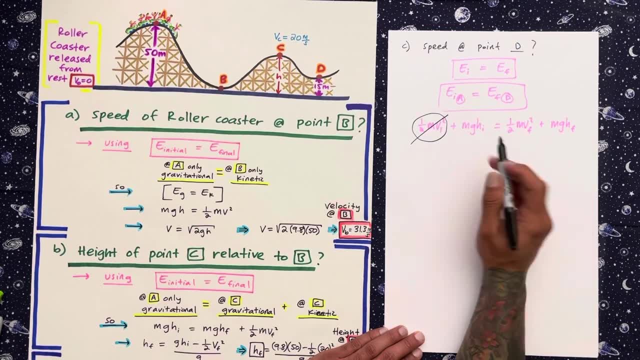 we have and we don't have. so again at point a right, we know that velocity initial was zero, so this is our initial and we're going to do the final one-half mv squared plus mgh initial goes to zero. right, velocity initial zero and we do have a height, so that stays. 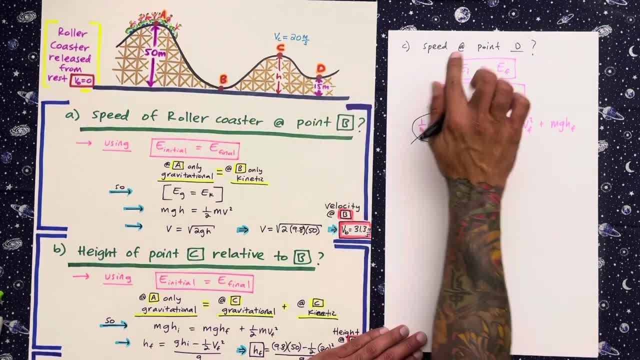 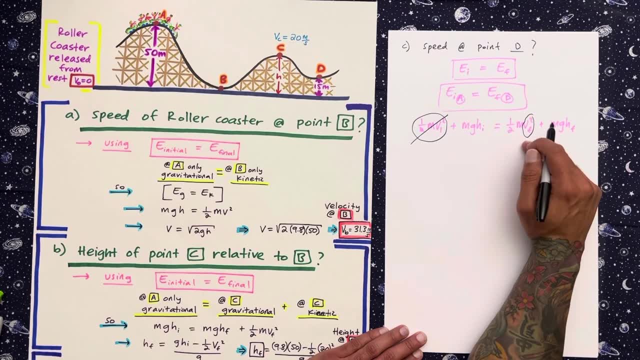 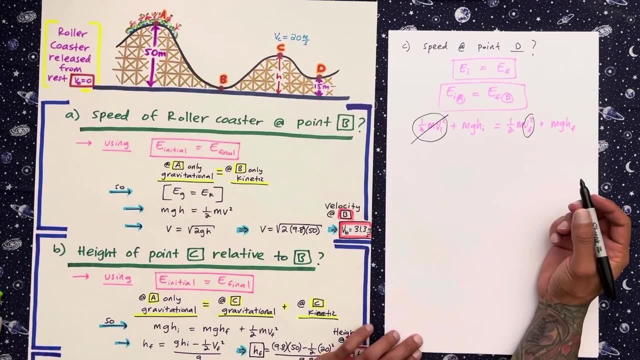 velocity final. well, that's what we're looking for, because that's the speed at point D. so this right here, velocity final, is what we're looking for. and MGH H, height final. we do have a height final ID, so we have everything we need. so now, 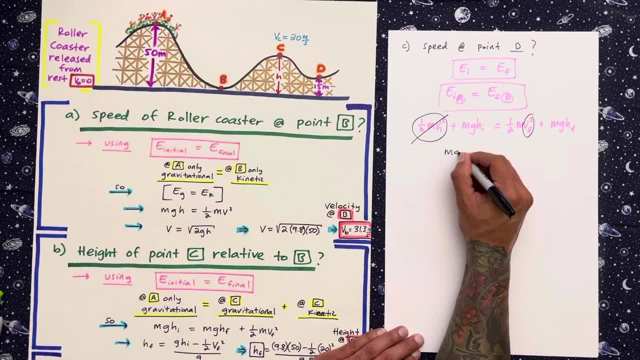 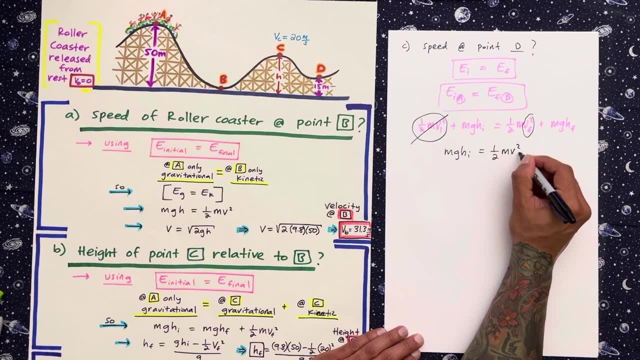 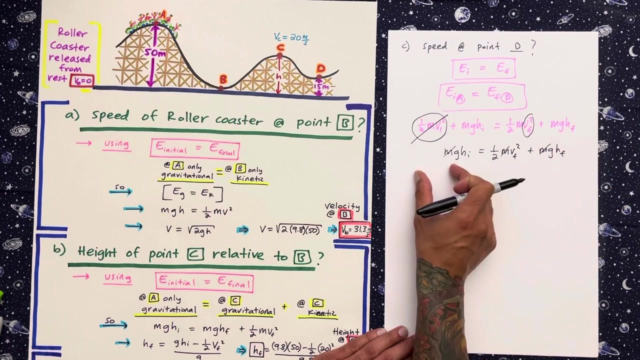 let's bring it down. we have MGH initial is equal to one half MV square final plus MGH final. okay, let's cancel out the M's and we're solving for velocity, final right. so let's take this and move it to the other side. all right, I'm gonna. 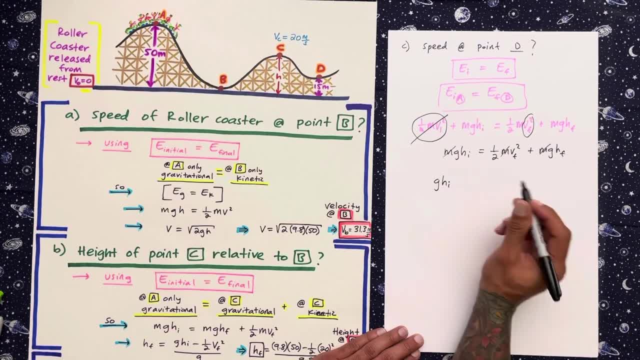 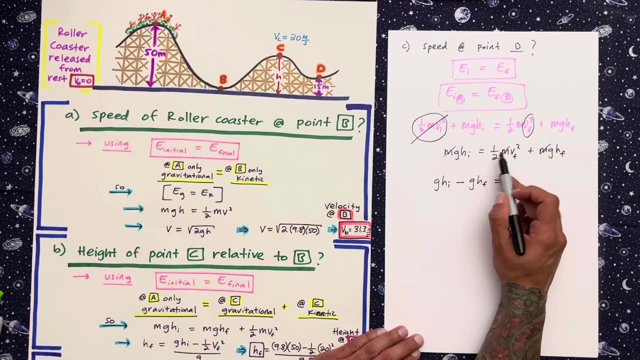 rewrite this gravity height initial, then I'm gonna move this over to the other side of the, the equal sign, so it becomes minus because it's positive right. so G- gravity height final right equals. now what's left on this side of the equation is this here, which is one: 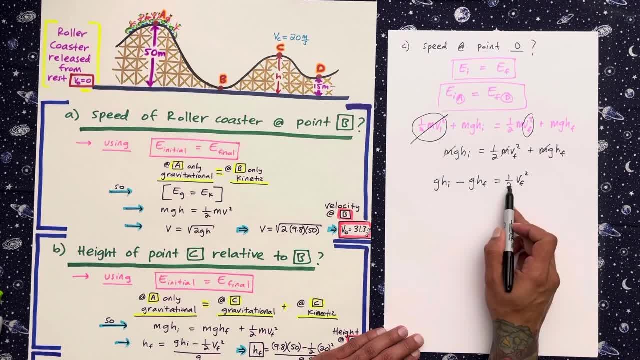 half velocity, final squared. all right, let's get rid of that two. so we're gonna multiply the two to the other side. so I'm just gonna put two in parentheses because it goes to the top of the equation, and then I'm gonna move this to the top and then I'm just gonna rewrite everything that we have here. 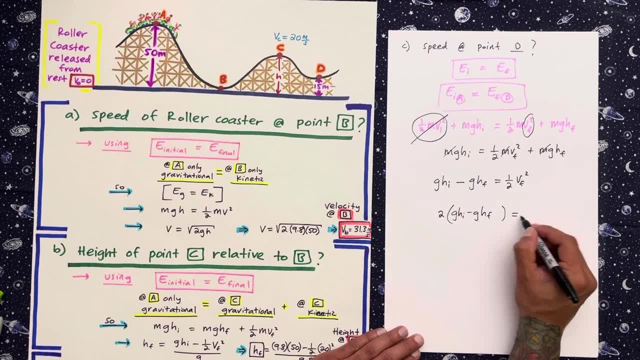 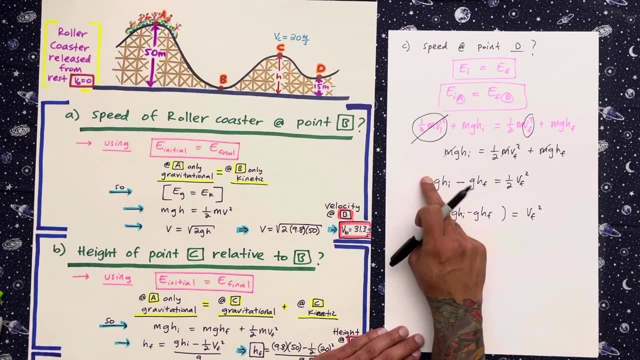 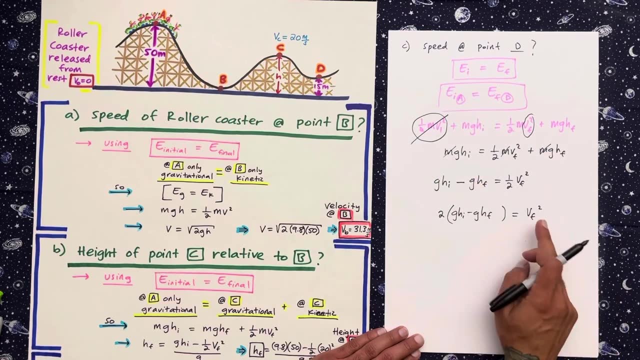 right. height. final equals velocity, final squared. so what I did was multiplied. so the two is on the bottom here. multiply it to the top on this side right, and so then I put it in parentheses so it can distribute back into both. okay, now all we need to do is take the root. so let's take the root both sides, so the final I'm. 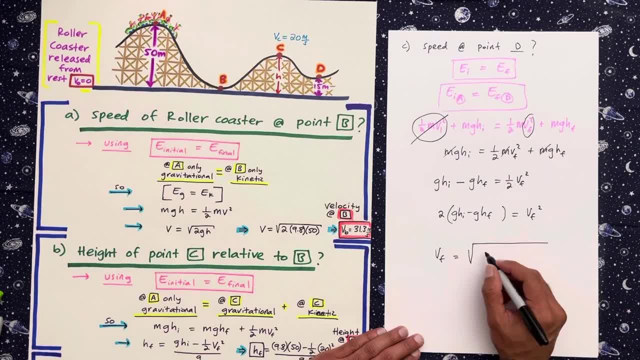 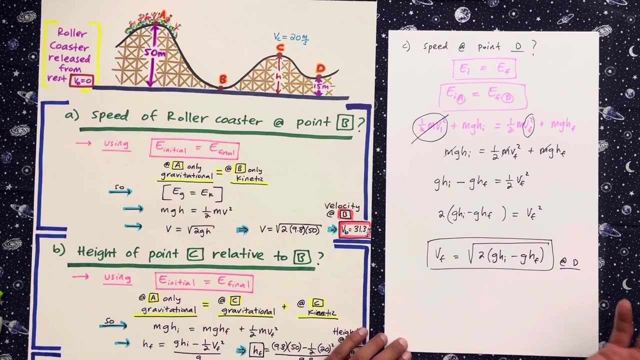 gonna write it on the other side- is equal to the square root of, and just write everything that's there. so everything that's there, okay, so the square root, both sides, to get rid of that. that's two. and now we have the velocity final at D. right, this is at point D, okay, and we have all the. we have. 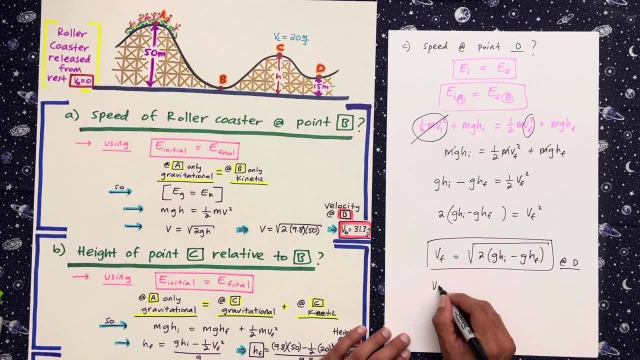 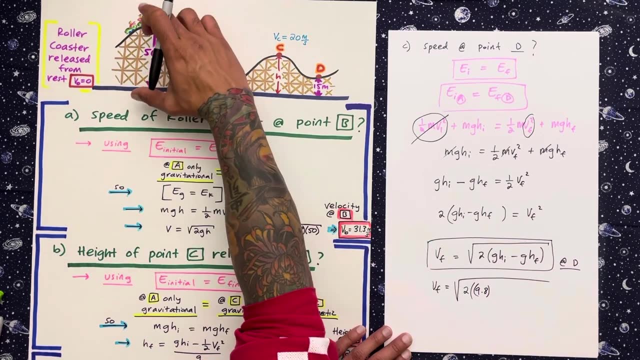 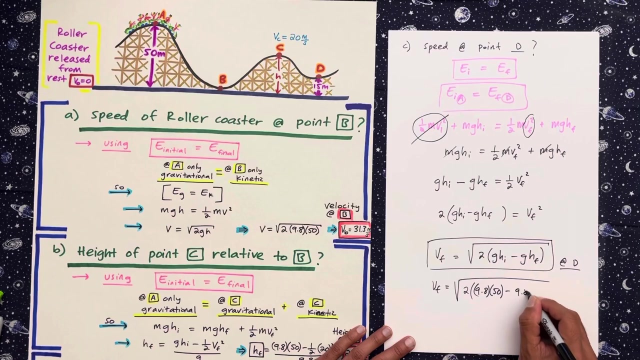 all the variables, all the numbers for this. so let's figure this out. velocity, final right, is equal to the square root of two. you know. gravity, it's nine point eight. height, initial of the initial energy. so don't forget that the initial energy, which is gonna be fifty minus nine point eight for gravity and height, 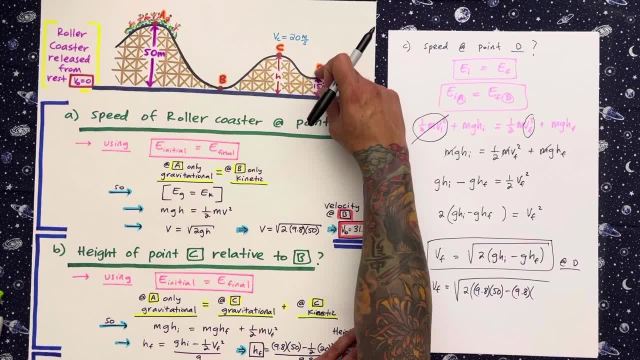 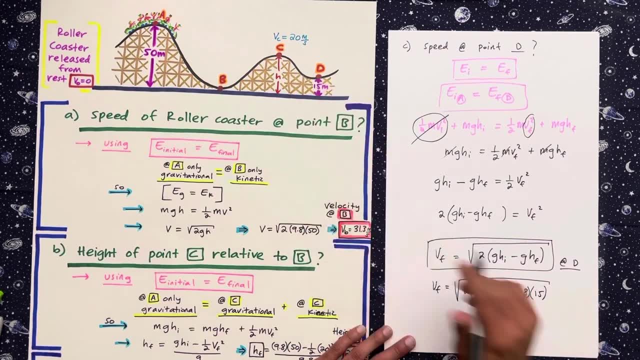 final, which is the point of interest, which is D, the height is fifteen, okay, so we're gonna have to do a little bit of math and make sure everything is in meters. so everything's good, and that's it. so now, putting this into the calculator, we get that velocity. final, at point D, is gonna be twenty six. point two: